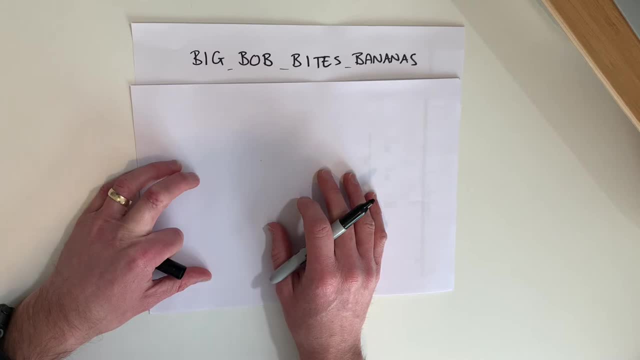 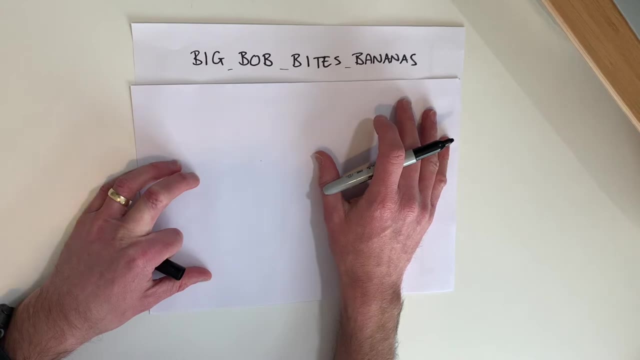 Now the first thing we need to do when we are looking at compressing this string of text is find the frequency of each character, and the goal of the Huffman tree is to find the shortest possible representation for the most frequently repeating parts of the text, or the phrase that. 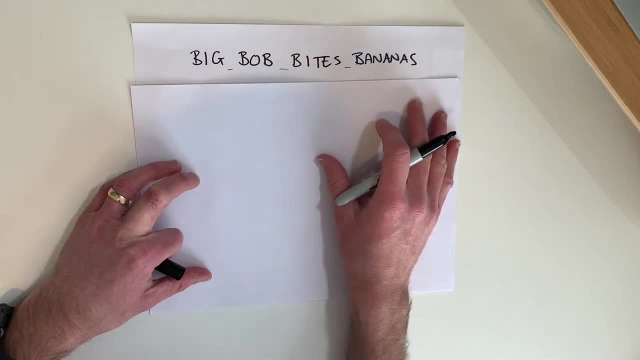 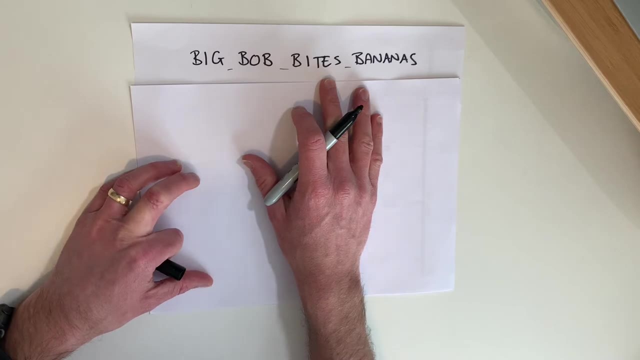 we are encoding. However, if something only comes up once or twice like this- E only appears once, we can get away with a fairly long representation for that, because we're not going to be repeating it in our text very often. So we're going to need to look at for each character what is the frequency. 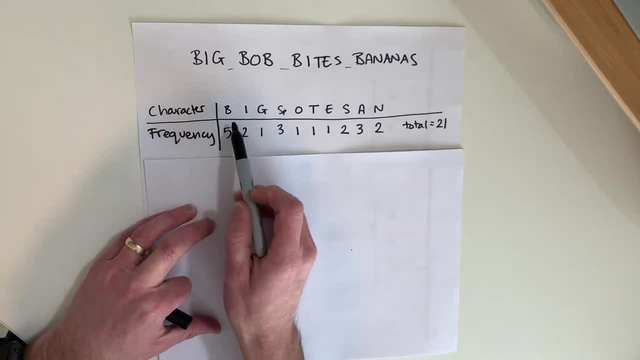 and I've got that here. So I just went through each character as it was. so I looked at the B. there were five B's, two I's, there's one G, there were three spaces. then we've got one O, one T, one E, two S's at Bites and Bananas. 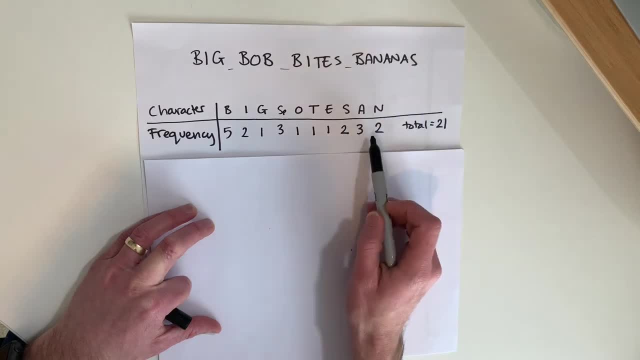 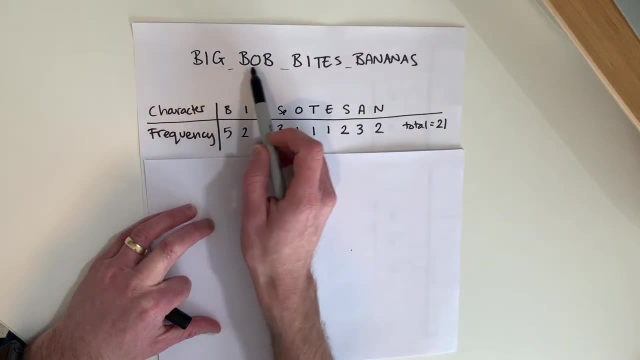 three A's, all in Bananas, and two N's, again also both in Banana, and the total there is 21, and that's a good little sanity check. you add those up. if you get the same length as your string, then you know you haven't missed any. Okay, so now that we've got our 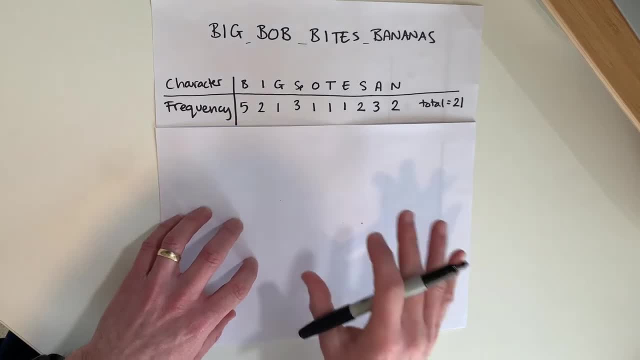 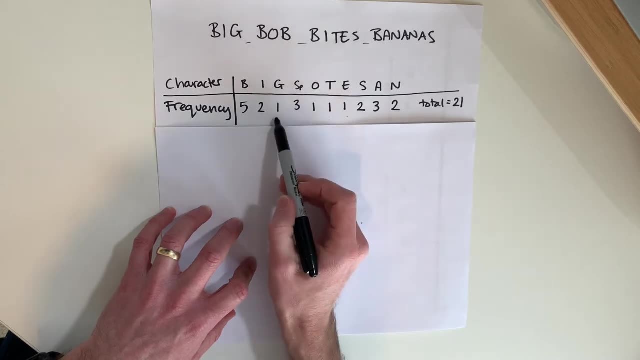 character frequencies. we can start building up our Huffman tree, and this is how we do it. we start off, we look through this chart and we find the items with the lowest frequencies first. okay, so G, O, T and E all have the lowest frequencies, So we're going to write those at the bottom of our 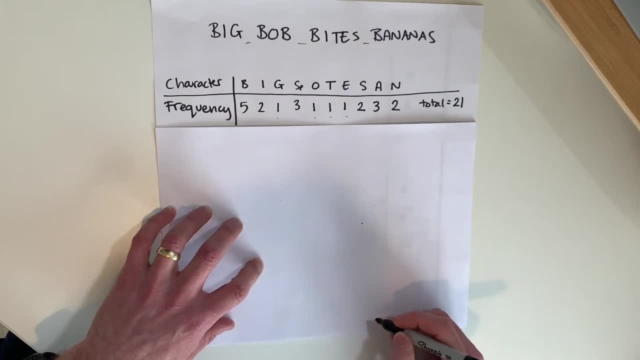 tree and we're going to give ourselves plenty of space. we start bottom up, so start in the bottom right and we're going to go. we're going to say we've got a G and so that's fine, we can cross that off. and we've got an O and we've got a B, and we've got a G, and we've got a B and we've got a. 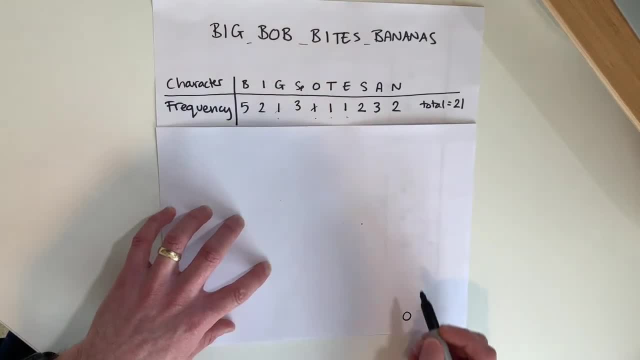 O, okay, and we've got a T and we've got an E- okay, and what we do is we need to combine these into pairs. so, starting at the right hand side, we build up pairs into a little tree, and what I mean by that is we connect them together and we work out their combined total. so in this case, the combined 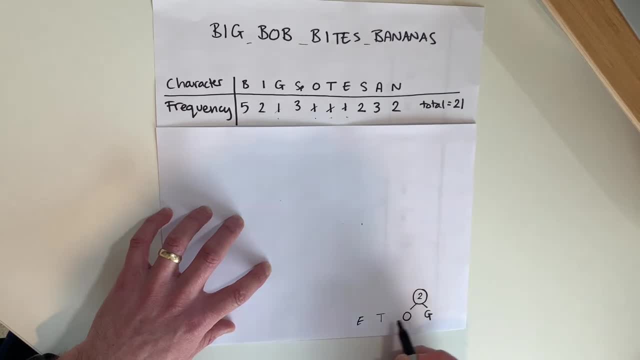 frequency of those two was two. okay, and then we go on to our next pair, where the combined total is going to be also two, because for each of these characters we had a frequency of one. now, if I had an extra, let's say I had five characters, all with a frequency of one, and I would just have 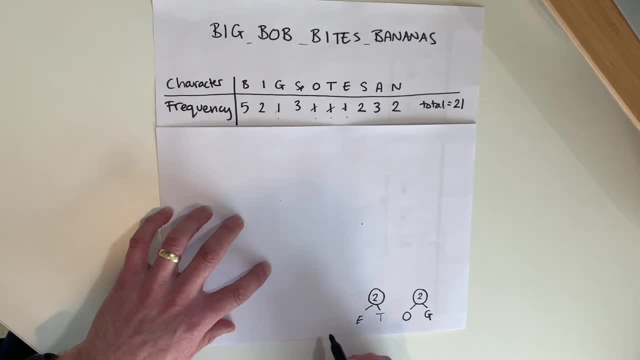 that here and I couldn't pair it with anything, so I just leave it for now. I just wait. we'd come back to it and you'll see an example of that in a minute. okay, so I've done my first, my lowest level of frequency, so I'm going to move on to my next level of frequencies, which are the, the I, which. 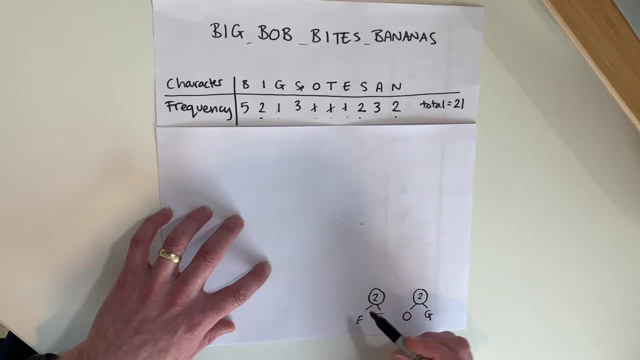 had two, S and N, all of which had two. now I'm going to write these physically and then I'm going to basically higher up in my um, in my little hierarchy in my tree. so, um, these were all like the one levels and now I'm going to put my two levels kind of here. so I'm going to start off. 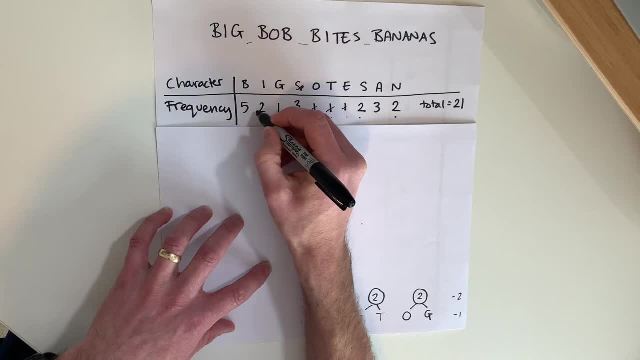 with my I. okay, so I've done my I. uh, what else did I have I? I had an S and I had an N. here's going to be our, our um unpaired item. and again, I'll do exactly the same thing. starting working sort of from the right hand side, I start pairing them. 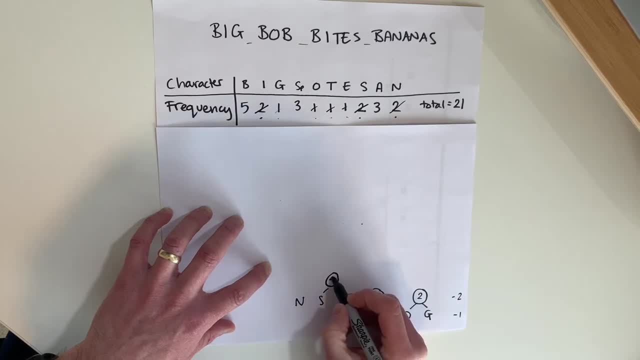 so S and I has a combined total of four and N. I just have to leave there for now because I haven't got anything to pair it with, okay, so let's go through and do the next level, and that's going to be my, my space and my A uh, which are both three. so I'm going to work it sort of like my next level. 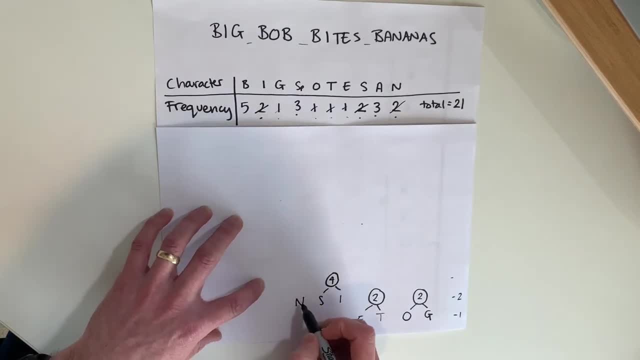 up, um. so let's see, let's go with space. so I'm going to put space here and that's that one and A. okay, so that's my A gone and uh, again working from the right hand side. I need to do some pairing. well, this N is still unpaired, so we're going to pair the N and the space. 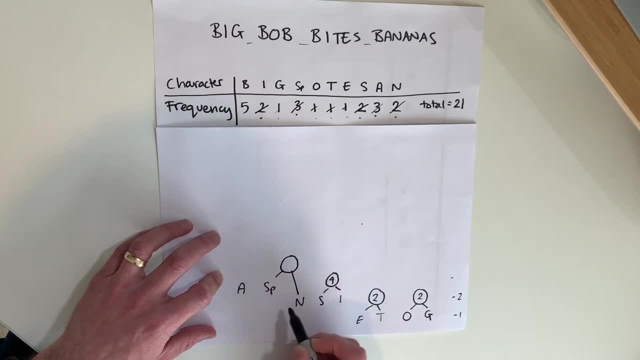 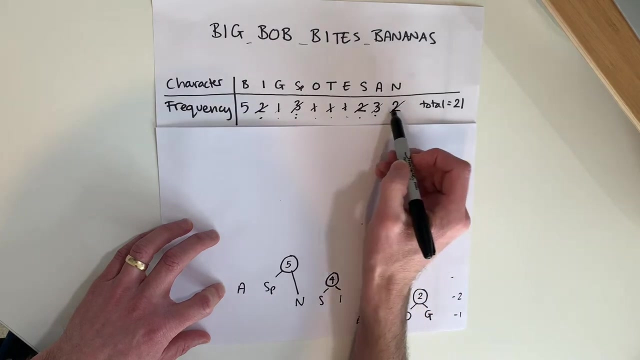 the combined total for that is going to be N was two, space is three, so it's going to be five, and the A is now unpaired. so we, you know, we just leave it there for now, and then we go to our next level, and then we're going to do the next level, and then we're going to do the next level, and then 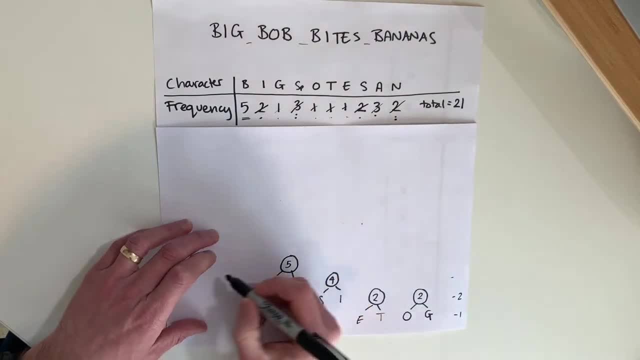 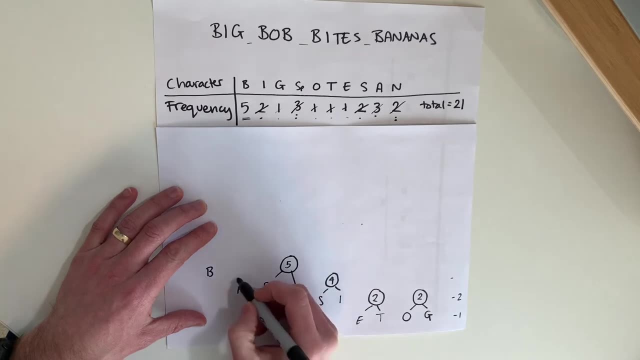 the only one we haven't yet done is, uh, the B at five. so I'm going to put a B up here and again. I've got to sort of combine now, uh, together, my A and my B, which has a combined frequency of five and three, which is eight. 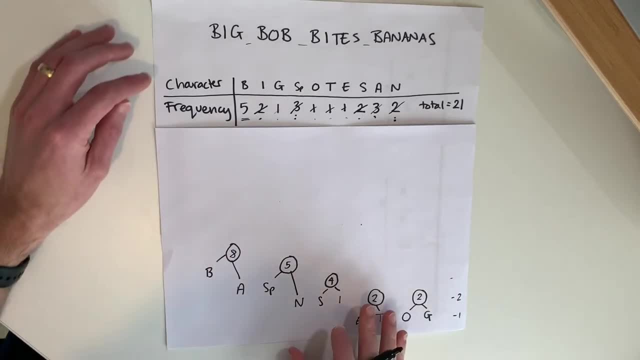 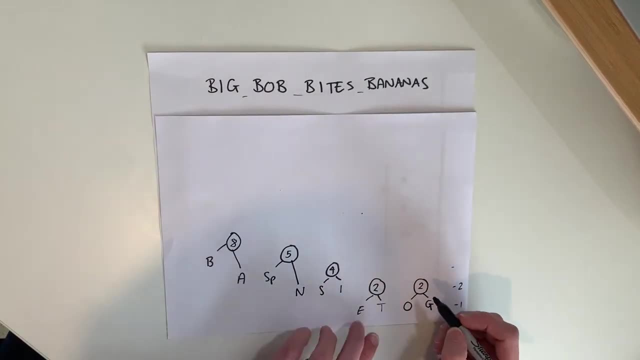 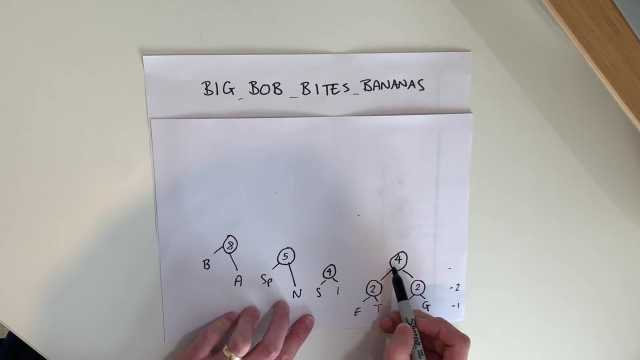 okay, so I've got all of my um characters now into my diagram. uh, now we just go right back to the right hand side again and we do another level of pairing. so two and two, we're going to pair those to a combined frequency of four. um, four and four, uh, I can do a combined frequency of eight. I could look at pairing, uh, these sides. 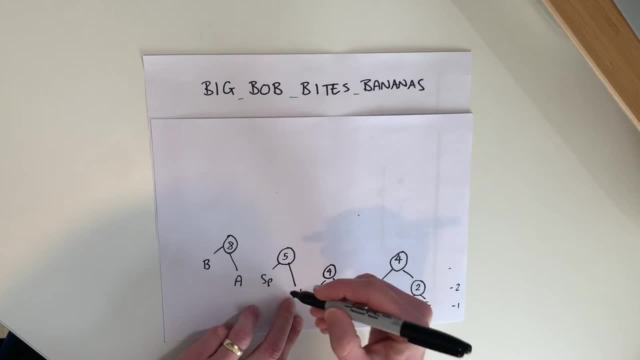 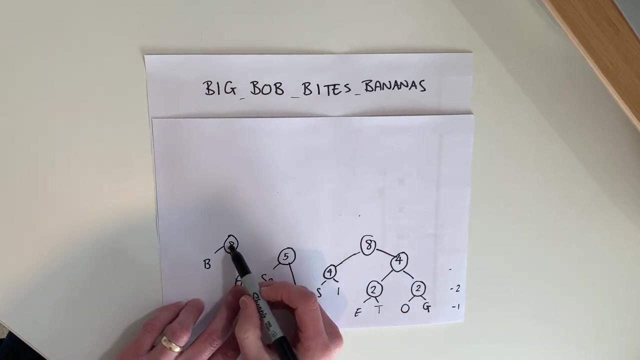 but, um, that would give me a combined frequency of nine and I want to go for the lowest combined frequencies that I can. so four and four gives me eight. okay, now I've got an interesting one, because this five I could pair it with this eight, or I could compare it with that eight. they're equal, um, but the premises always work from the. 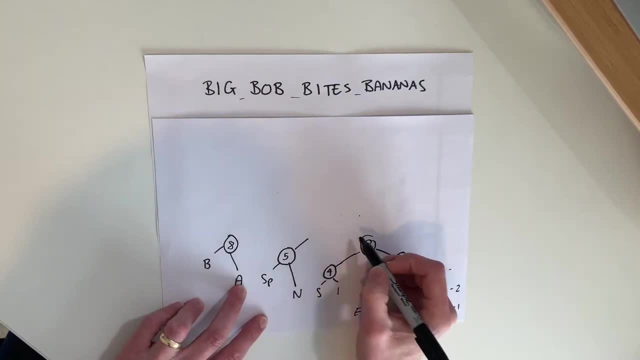 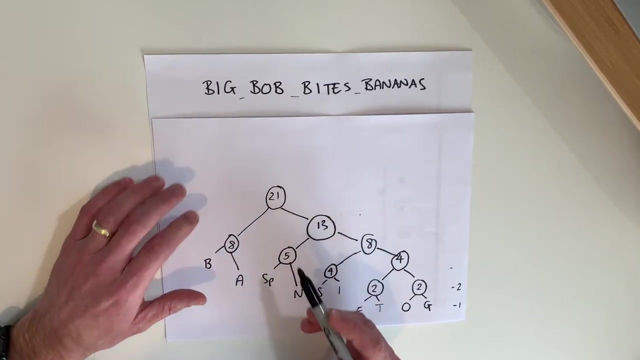 right hand side, so I'm going to- you know, I got here first, as it were, so I'm going to go- eight and five, which combined together is 13, and so my final pairing is eight and 13, which is 21, which again is our total frequency. if you remember, we had, uh, 21 characters in total, so we've created. 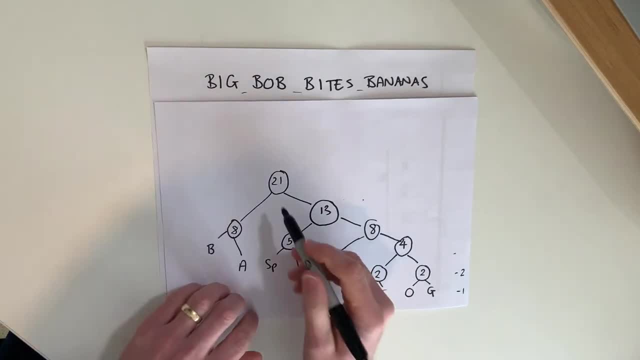 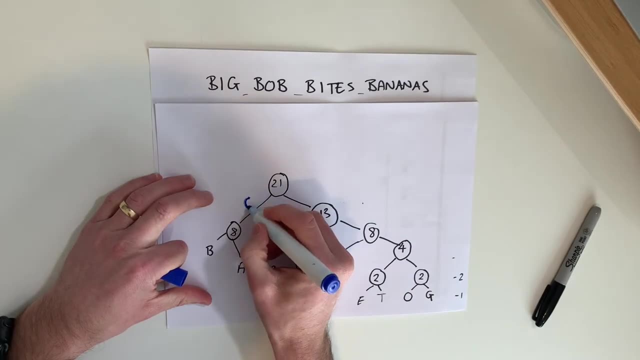 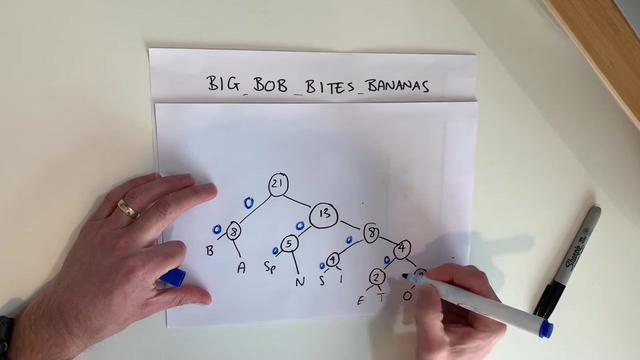 three, okay, fantastic. next thing to do is we need to actually label the branches, and this is really easy. all we do is every left branch we're going to label zero. so all of these are left branches where I go to the left from a node, and all of my right branches I'm going to label one. 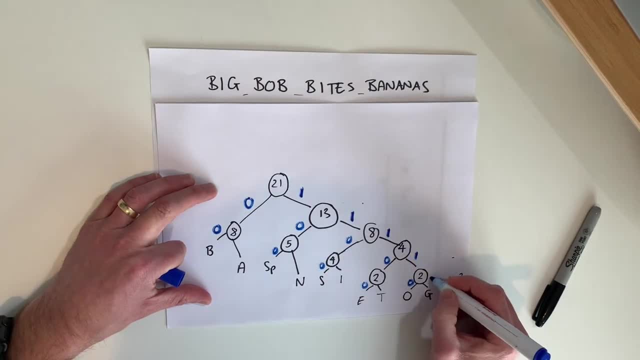 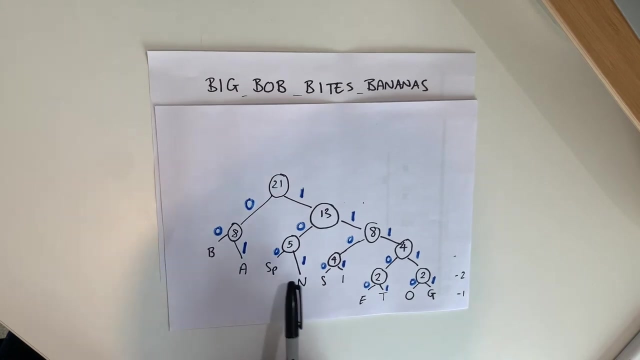 so that's all the way down the right. I've also got a right branch here. I've got a right branch here and a right branch here. okay, and from this tree I can now get an encoding for every one of these characters. so let's uh write that up, maybe at the top. so let's go for character and encoding. 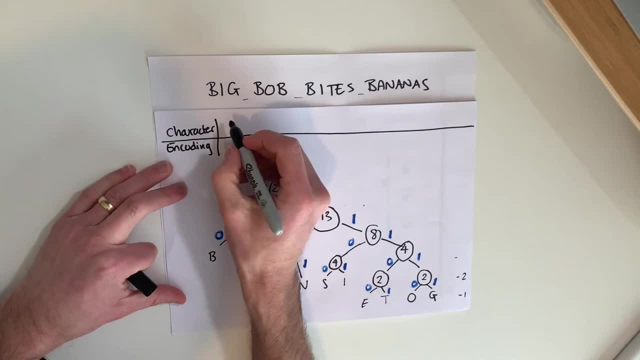 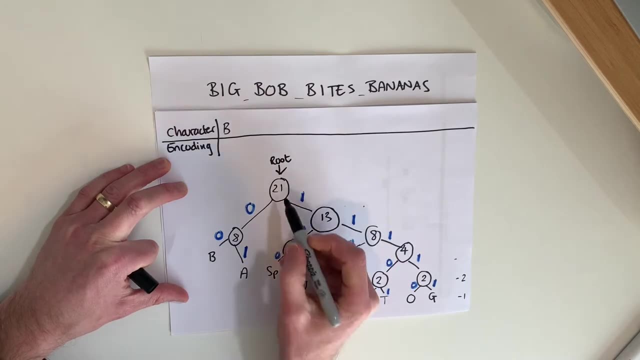 okay, and let's start here on the right hand side. so for the character b, our encoding we start at the root. this is our root, and we just work down the path that gets us to the character we're interested in. so for the b, it was zero, zero. so the binary encoding is going to be zero, zero. okay, then the a was zero one. 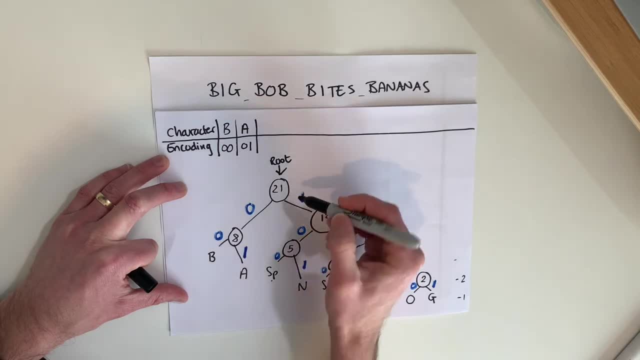 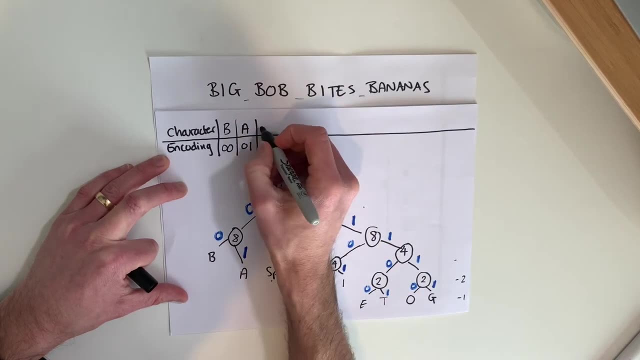 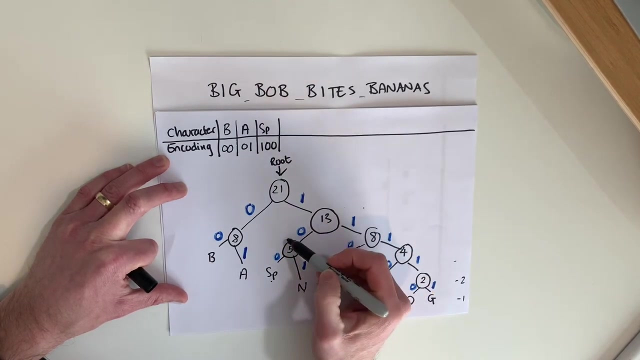 okay, then the next one we had was sp, which I went one. I had to go to the right, so one zero zero. so for sp, or space, it is one zero zero. for n, it is one zero one. for s, it's one one zero, zero. for i, it's one one zero one. 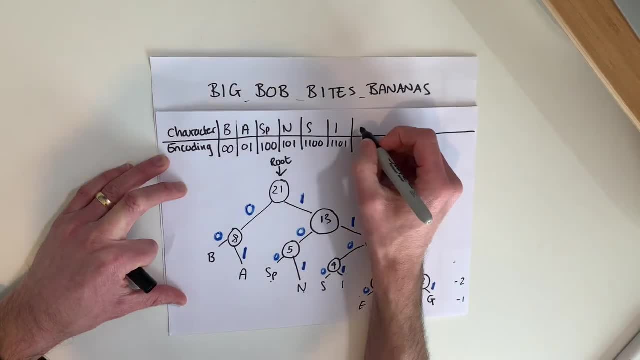 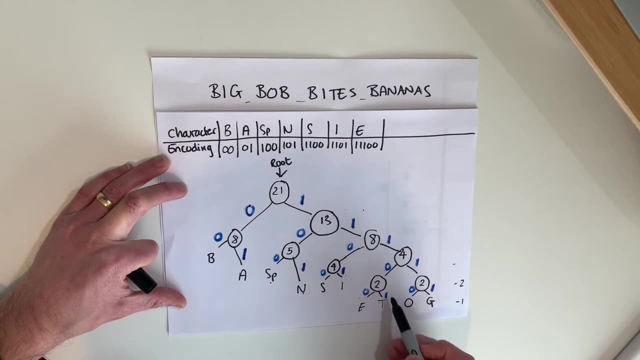 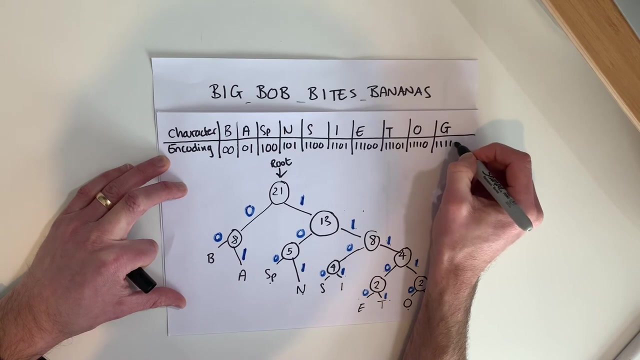 for e it's one, one, one, zero, zero. for t it's one, one, one, zero, one. for o it's one, one, one, one, o, or zero, I should say. and for g it's one, one, one, one, one. and that's our encoding for each one of our characters. 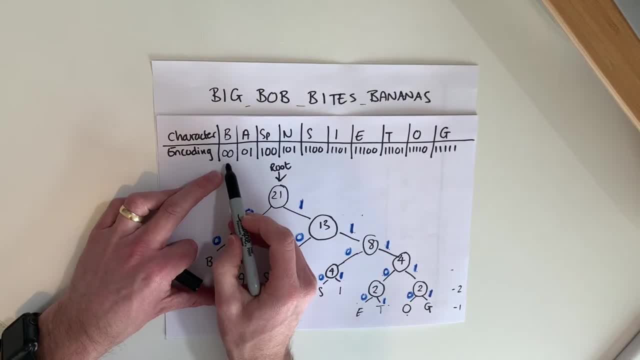 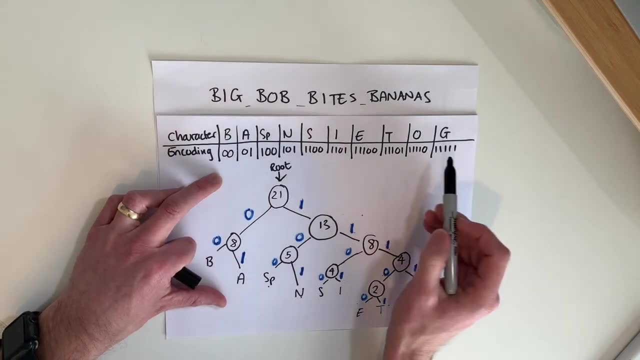 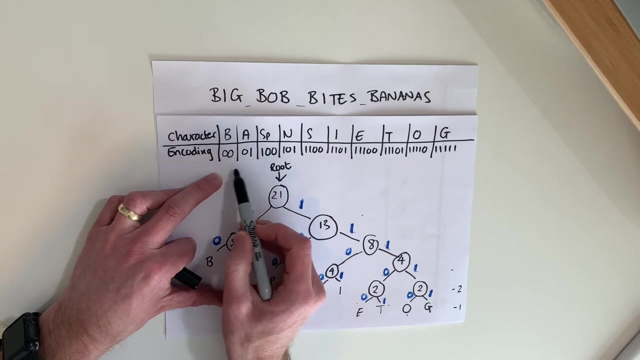 now notice, the principle has held that the most significant or the most frequent character has the smallest binary representation, whereas the least frequent characters have the longest representations. these are each going to take five bits to store, whereas uh b and a, the the most frequent characters, take only two. two bits each. 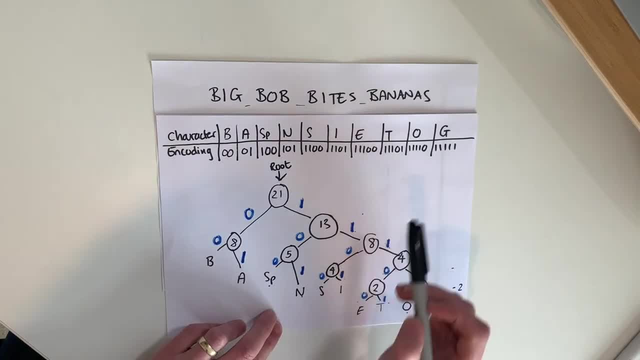 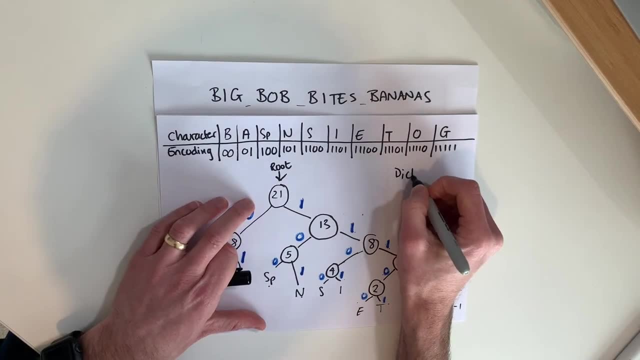 okay. so that's how we career our hoffman tree and how we create our encoding for each character from the hoffman tree, which we call the dictionary. so now that we've got our hoffman tree in our dictionary, we can now use the dictionary to 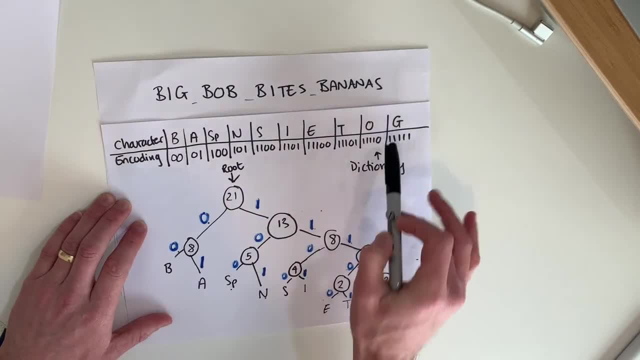 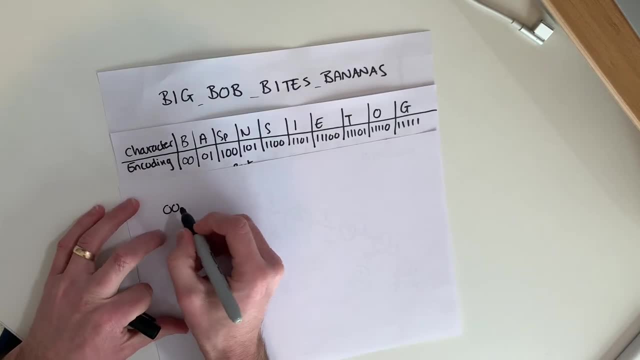 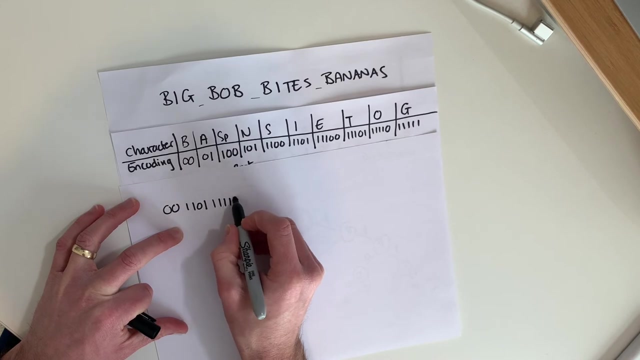 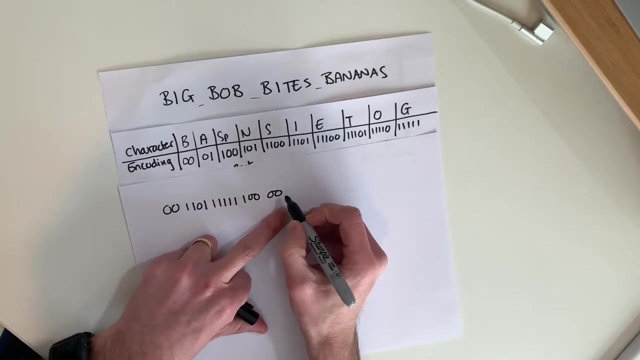 encode our original message using our dictionary representation. so big bob bites bananas is going to be zero. zero for b, big one one, zero one. g, 1, 1, 1, 1, 1 space 1 0, 0, and then Bob and so on. I'm going to complete this. 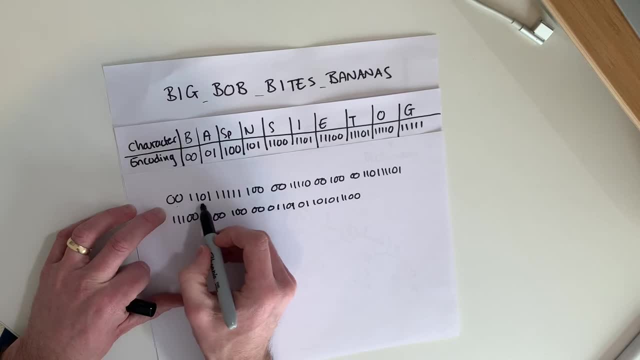 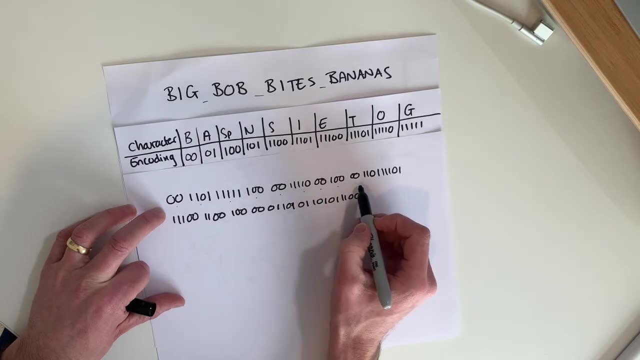 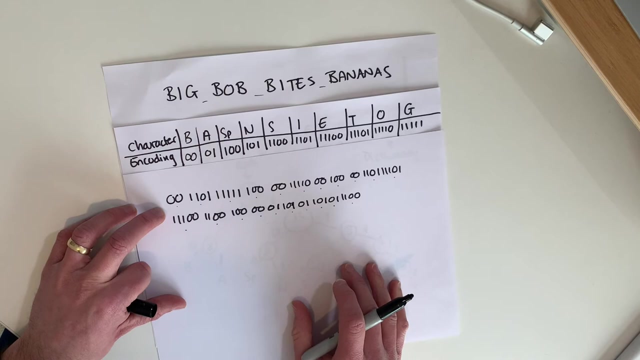 Okay, and there is our encoding. so that's my B O no B I G space. B O B space. Big Bob B I T E S space bytes B A N A N A S bananas. Okay, that's the encoding. So let's just look at how many characters- or sorry, how many bits we've used to encode that. 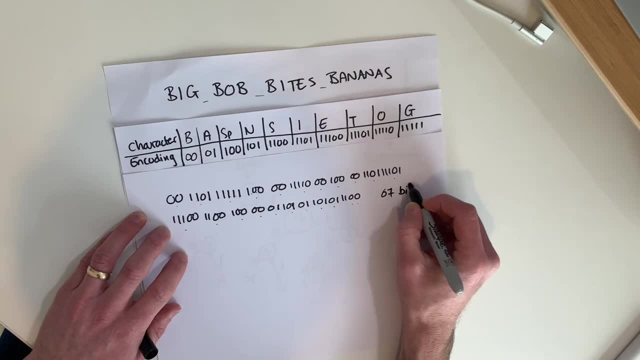 67.. 67 bits to encode our message. Now, if we think about using 7-bit ASCII, we're going to have to encode our message. So we're going to have to encode our message. 67 bits to encode our message. Now, if we think about using 7-bit ASCII. our original message had 21 characters, if you remember. So if we had 21 times 7 bits per character, if we're assuming basic ASCII, that would be 147 bits for the original, but only 67 bits compressed. As you can see, that's a significant reduction. 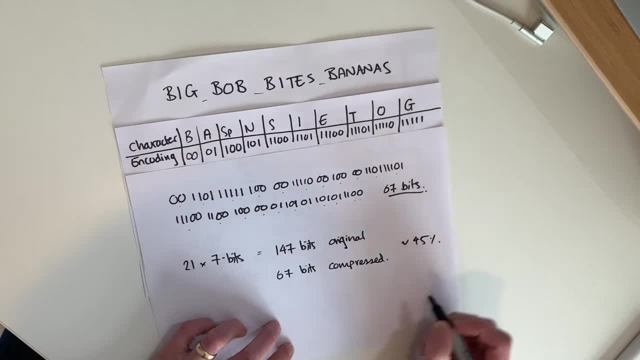 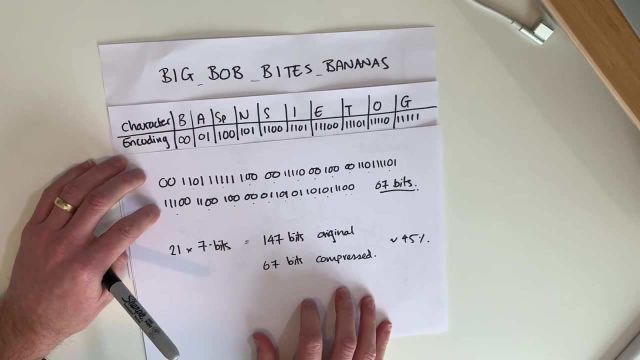 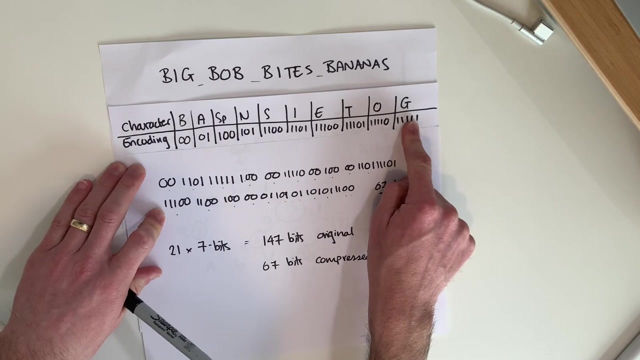 of about 45% of the original size. Now it's not quite as simple as that, because in reality, we have to also transmit with our encoded, compressed data. we have to encode our dictionary as well, So we're obviously going to need a byte for every character we send, because 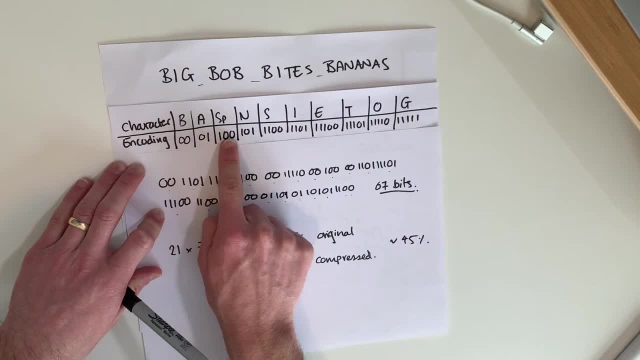 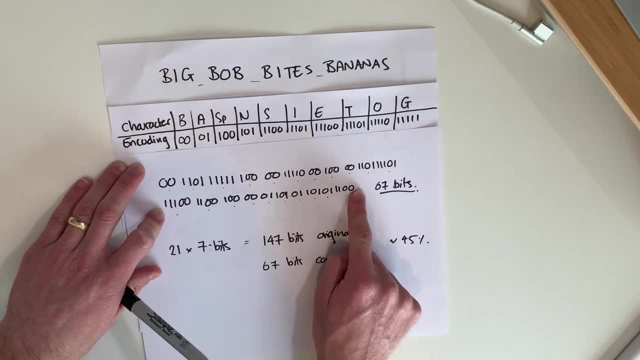 we need to know what it translates to at the other end, plus the variable number of bits for each byte. So all of that data needs to be sent. You can see, here we've got a lot of cells and then we've got one and we've got a lot. 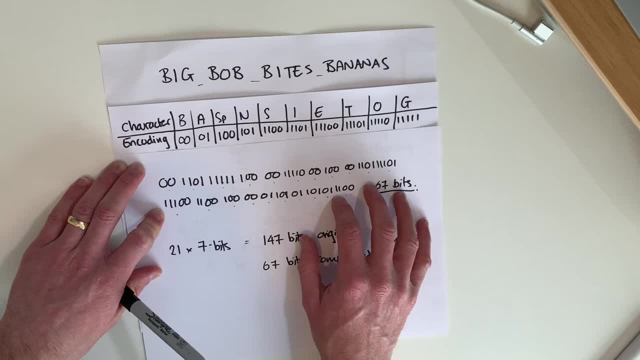 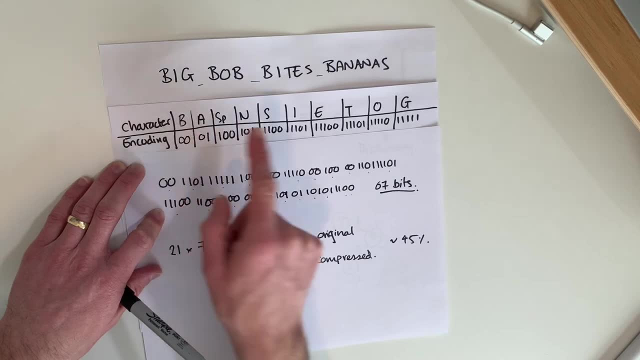 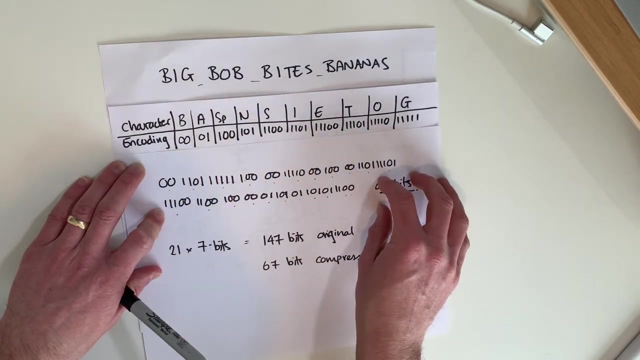 of cells. So let's do, or we can do, this one. So we're going to say that we want each cell to have a certain number of bytes so we can actually take away the number of bytes. So that works. And here you can see that it has all the buttons. So it's all the terms and 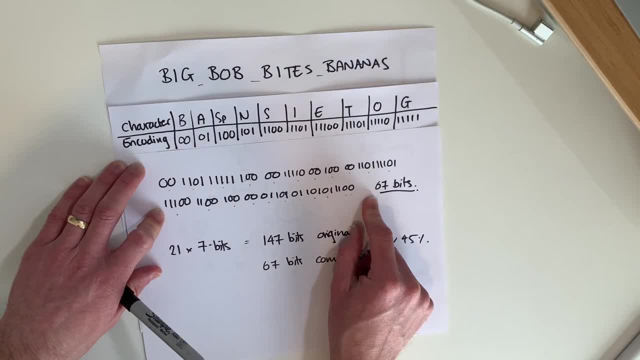 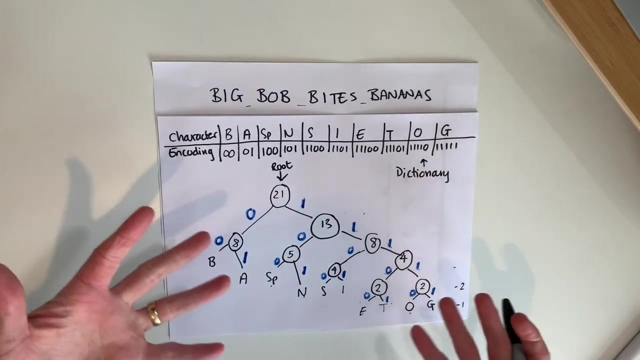 you know, in a much more efficient format, And you end up with a dictionary that is proportionally not that big compared to the message that's being sent, And that's where you get your greatest encoding benefits. Now we need to see how would we actually use this to decode a message? 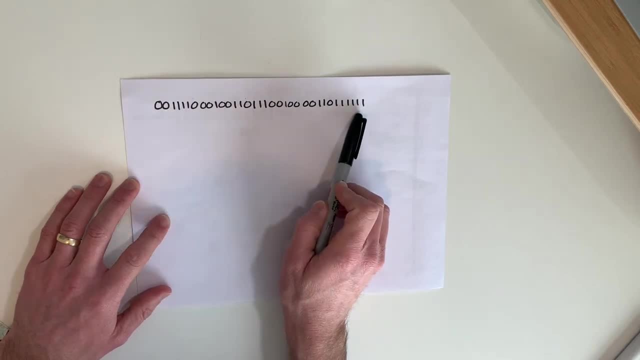 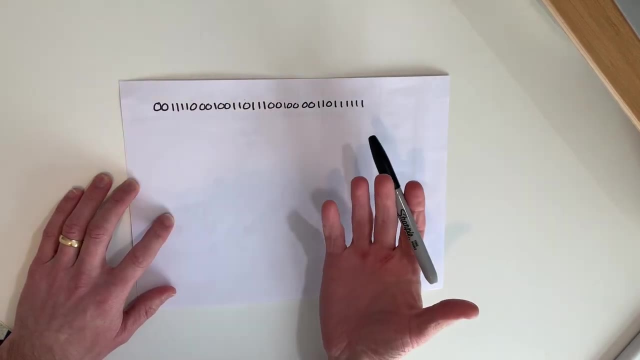 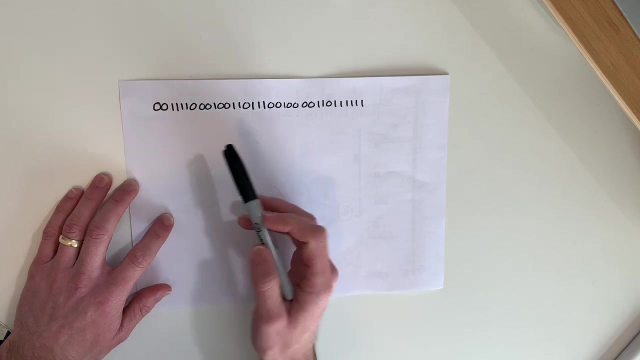 Okay, so here is my binary string that's been encoded using this Huffman tree, And we need to decode that into a message. And one of the first things you'll think is: I don't even know when a character starts and ends. There's no obvious way of knowing it's because they're not fixed bit. 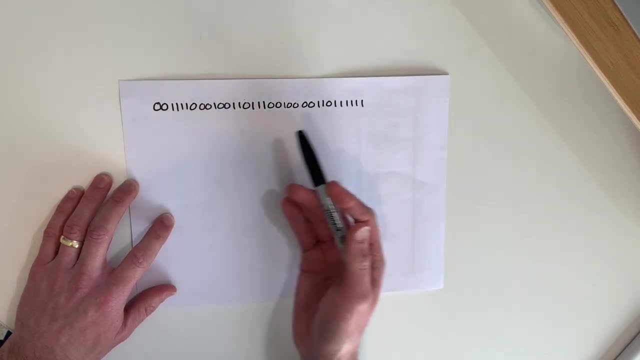 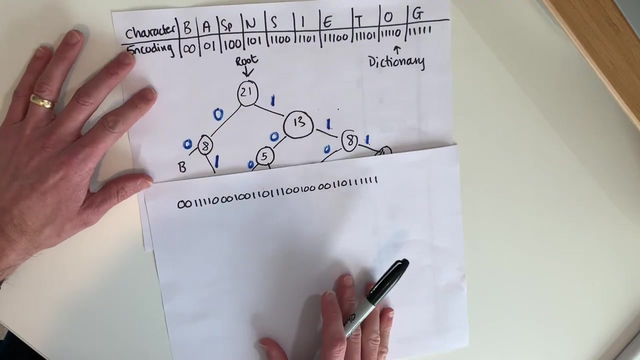 widths. So it's not like we have seven bits per character like we do in ASCII. We could have two bits for some characters. we have three bits for other characters. So how on earth are we going to break this down into a meaningful string? Well, let's go through it and show how it works. 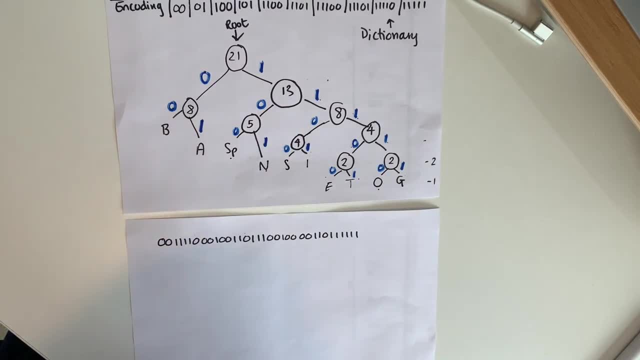 It's actually surprisingly easy. All you need to do is you start at the beginning of your string And you go to your root And you just follow all the bits through until you hit a character. we call that a leaf. So let's start here. So I've got a zero. So if I go to my root, 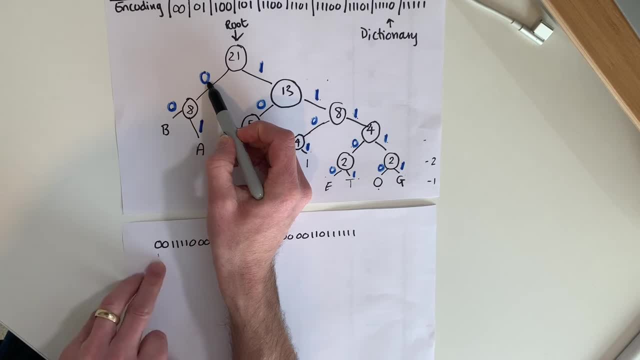 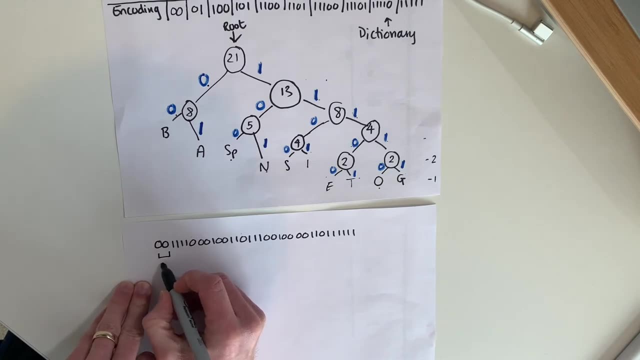 and I go to zero. I get here, So I'm not at a character yet. But then I've got another zero which gets me here, And that does get me to a character. Zero zero gets me to the B. This zero zero is a B, So let's now try the next one. So I've got an. I Sorry, I've got a one. 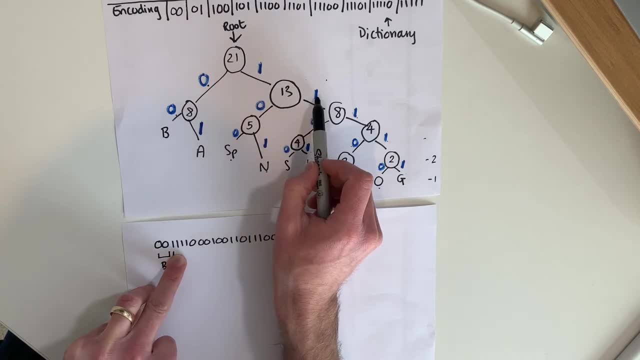 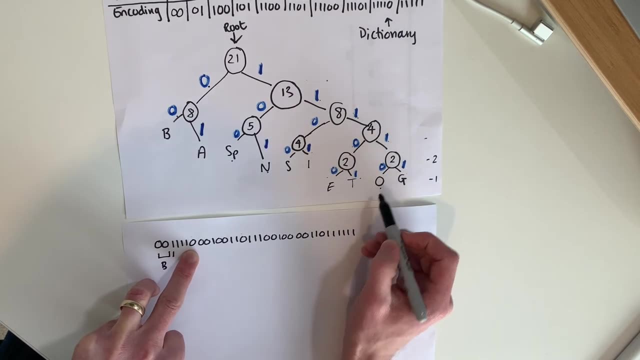 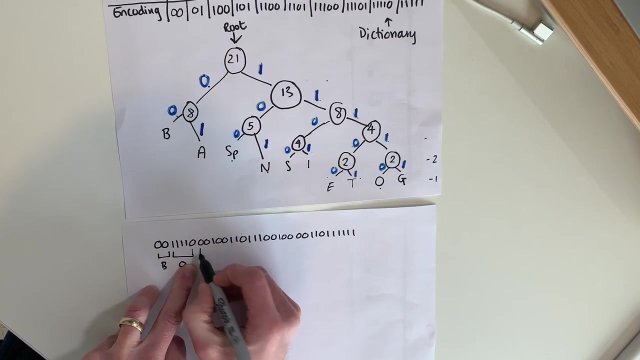 even One another, one another, one another, one, zero. Ah, that's got me to a character, So that must be where I finish. And that's an O and that's a bob. So now let's start my next one. I start. 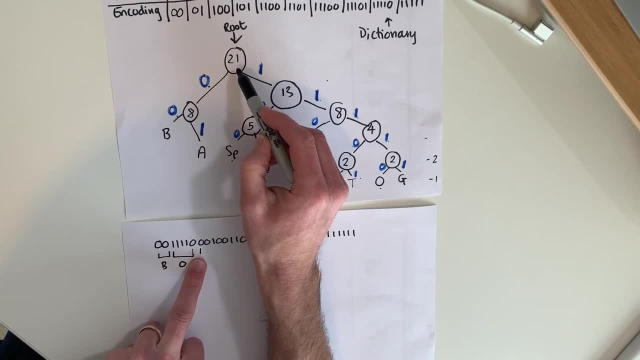 right back up to the top And I'm on a zero again, Which gets me here. Another zero gets me here. So that gets me to back to that B. So I start again at my root with a one. So I go one, zero, zero And I've landed. 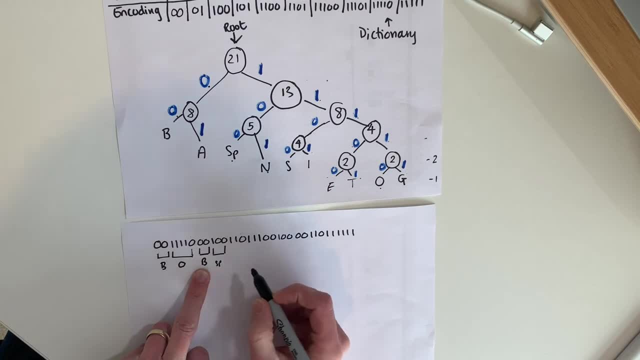 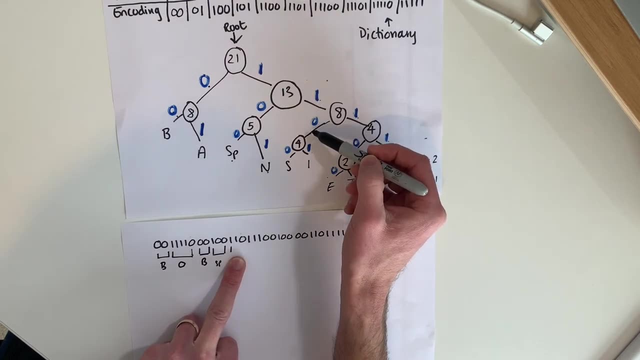 at a space, So this must be a space. I'm back here at this one, So let's start again. Root, let's go. one, Okay, one. It's got me here. Okay, zero, Yep, One gets me down here to an I, So this.